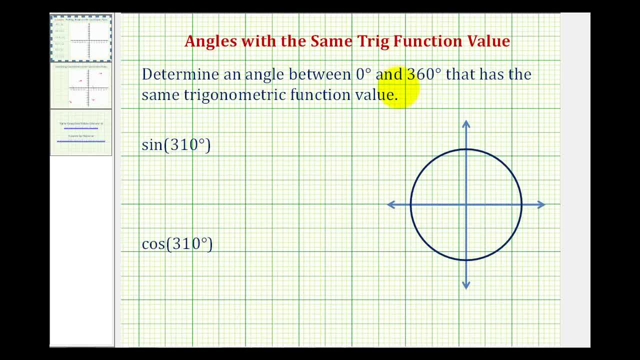 We want to determine an angle between zero and 360 degrees that has the same trig function value as sine 310 degrees and cosine 310 degrees. Well, sine theta is equal to y over r and cosine theta is equal to x over r, Where x and y would be the point of intersection. 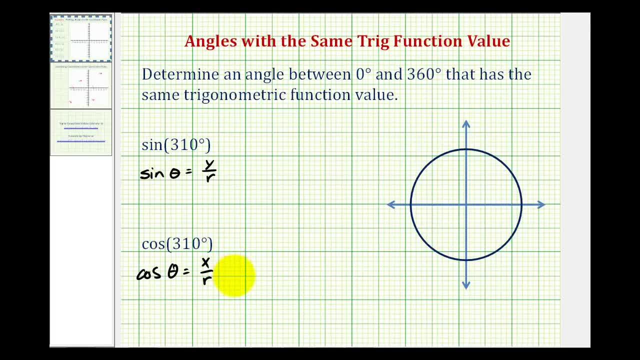 of the terminal set of the angle and a circle centered at the origin with radius r. So let's go ahead and sketch our angle of 310 degrees- Here's the initial side- and then we rotate counterclockwise, 310 degrees. Well, this would be 270 degrees. 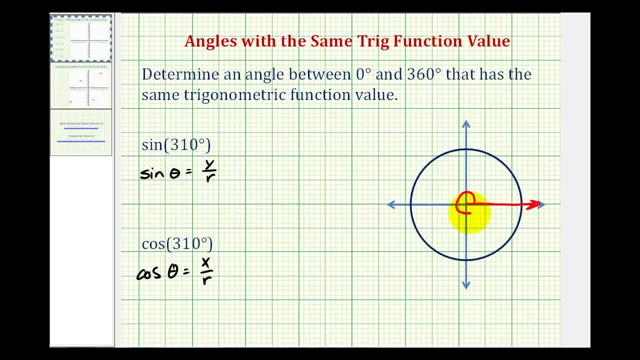 So we need to rotate 40 degrees more, maybe somewhere in here. So the angle might look something like this And notice how the reference angle would be 50 degrees right here, And then this point of intersection here can be used to determine the trig function values. 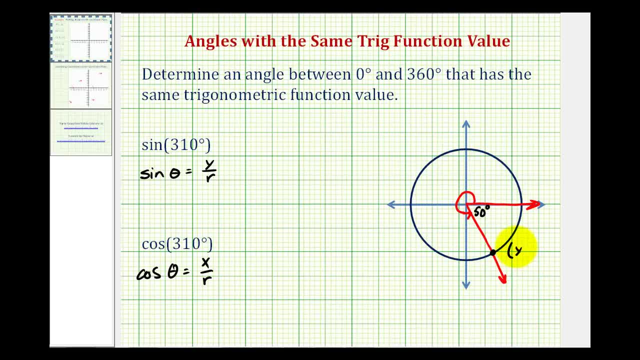 Notice how the x-coordinate would be positive and the y-coordinate would be negative. Then the radius of the circle would be the length of this segment here. Now, if we want to find another angle between zero and 360 degrees that has the same sine function value of sine: 310 degrees. 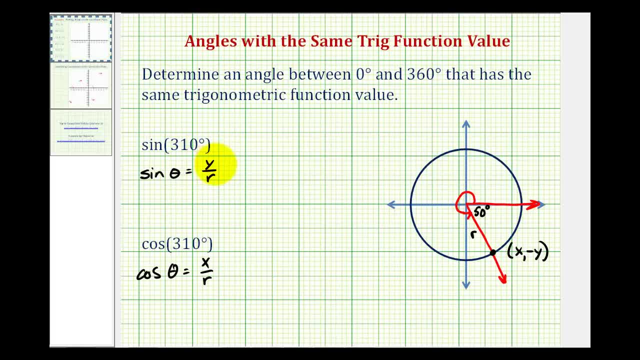 notice how we need to determine another angle where the y-coordinate would be the same as this point right here. Notice how the x-coordinate is not involved for the sine function. Well, we know the y-coordinate is going to be negative in both the third and fourth quadrants. 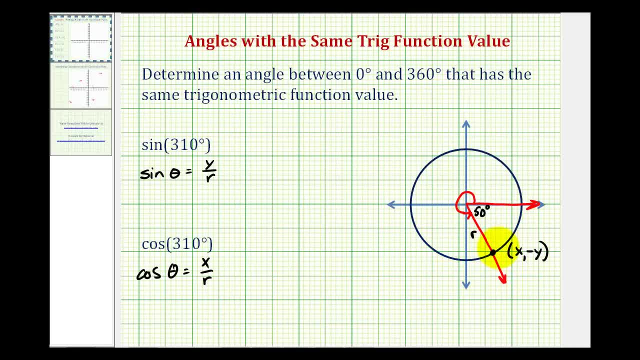 So we need to find another point on this circle that has the same y-coordinate of this point. It looks like it would be somewhere over here, Which means the terminal side of another angle that has the same sine function value as sine 310 would have to pass through this point here. 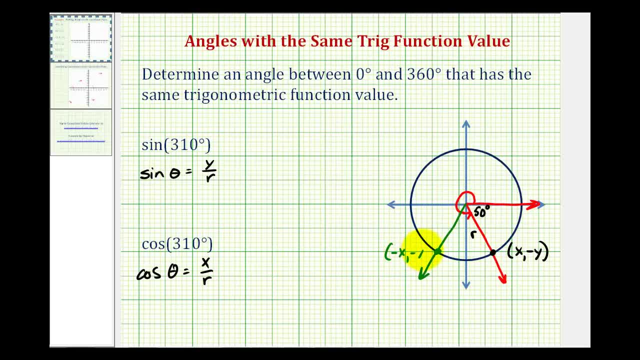 So this point would have the coordinates negative x, negative y, But it's also going to have the same reference angle. So this angle here would be 50 degrees. So the angle that we're looking for that has the same sine function value would be this angle here.